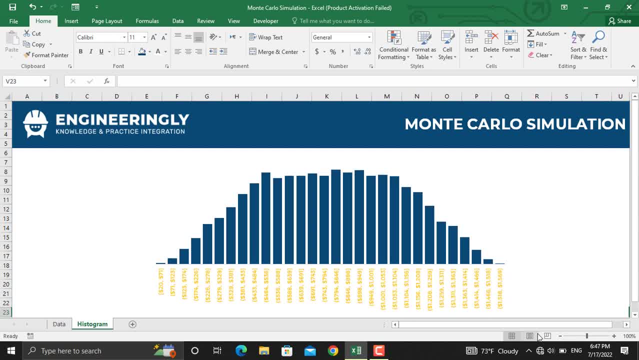 and how is it used for quantifying the risks in a project? Monte Carlo simulation performs risk analysis by building models of possible results, by substituting a range of values. Every decision has a degree of uncertainty. A Monte Carlo simulation helps you get more information. It allows you to 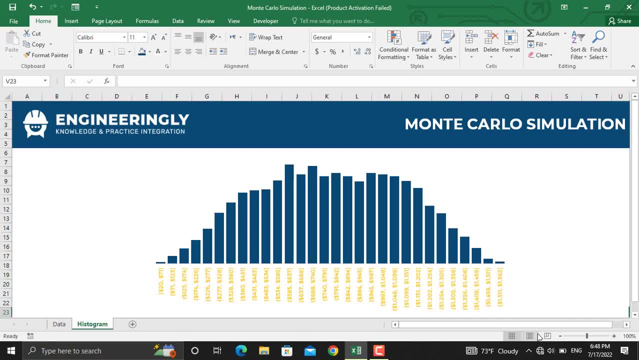 make sound choices and avoid surprises. later You can run this simulation to analyze the impacts of the risks on cost schedule and other constraints of your project. In project management, Monte Carlo analysis is a risk management technique used to conduct a quantitative analysis of the risk. 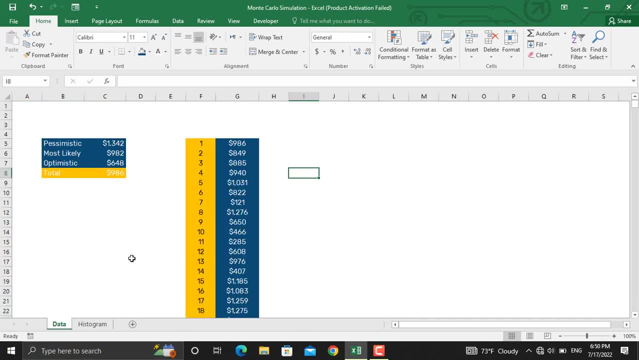 In order to create this model, I have used the data for 10,000 different probabilities. I have the pessimistic cost for my risk, I have the most likely cost for the risk and I have the optimistic estimation for the risk. I have used a P-E-R-T method in order to have a total value for all the 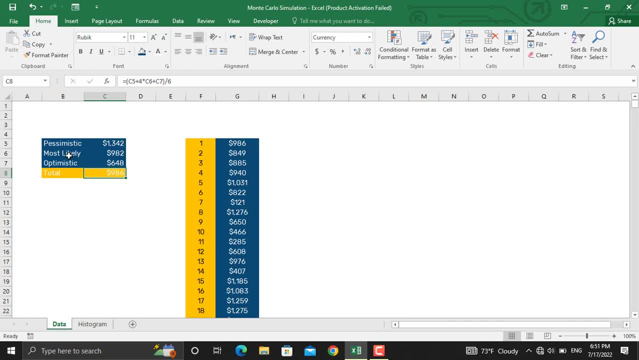 scenarios in here: Pessimistic plus four times most likely plus optimistic, divided by six. And again in here: if I press the F4 key, as you can see, all the information in here will be changed And I have a list of 10,000 different probabilities in here. In today's video we will discuss how to prepare. 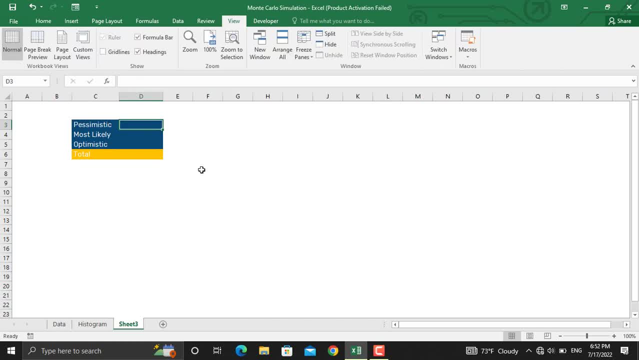 such models using Microsoft Excel. In order to have values for pessimistic, most likely and optimistic, we should insert random values into here. For example, for the pessimistic we will have a value between one thousand dollars and one thousand five hundred dollars. So I'll write down equal sign ran. 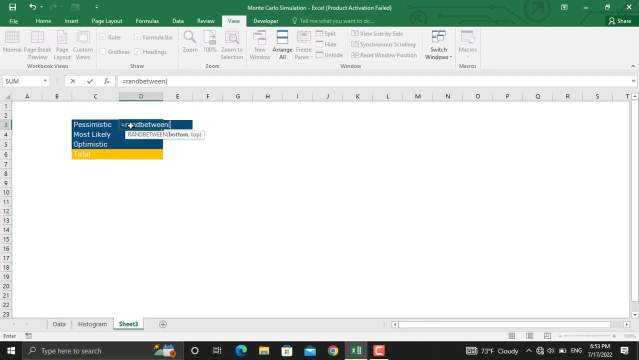 between a value of one thousand up to two thousand. I'll close the parenthesis and press enter. It will give me a random value. For the most likely, I'll write down a value between five hundred and one thousand US dollars. So again, I'll write down: ran between. 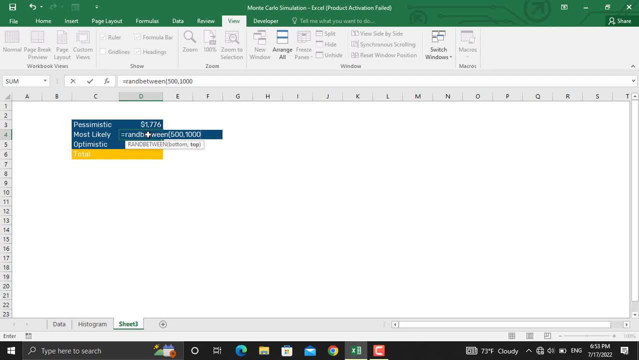 five hundred and one thousand. I'll close the parenthesis and press enter. And for the optimistic I'll have a value between zero and five hundred. So again in here I'll write down: equal sign ran between zero and five hundred. I'll close the parenthesis and press enter For the summation. 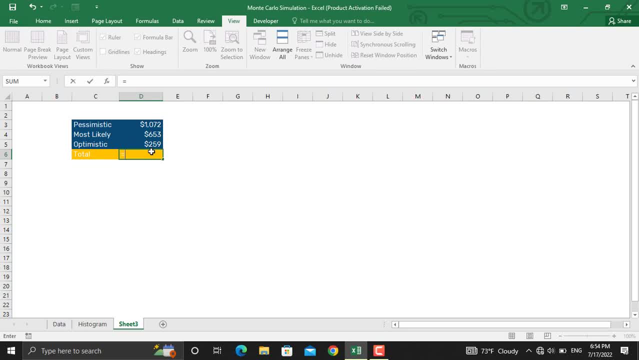 again. I will use the PERT method, So I'll write down equal sign, open the parenthesis- pessimistic value plus four times most likely plus optimistic, and I'll close the parenthesis and divide this by six Now in order to have different probabilities for our risk cost. 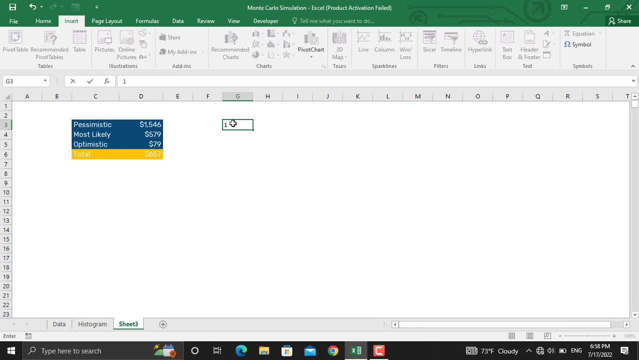 I'll use ten thousand different probabilities For that. I'll write down one in this cell and then I'll fill the other cells automatically. To do that, I'll go to home from here, I'll go to fill and in here I'll click series. 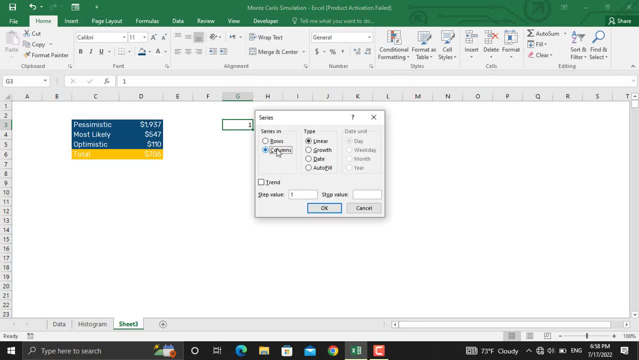 From the series. I'll click columns and in here I'll write down the stop value as ten thousand and then click ok. It will be automatically filled. For the cell number one, in here I'll write down equal sign and equal it to this cell Now in order to automatically fill the other cells with the. 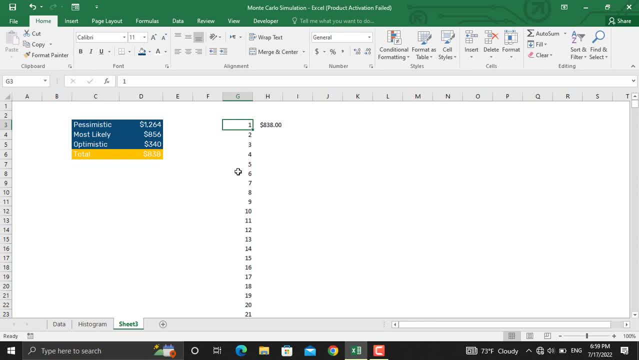 probable values. I will select the cells containing the numbers and the cells containing the values for the risk. I'll hold ctrl shift and press enter Now in order to automatically fill the other cells with the probable values. I will select the cells containing the numbers and the cells containing the values for the risk. 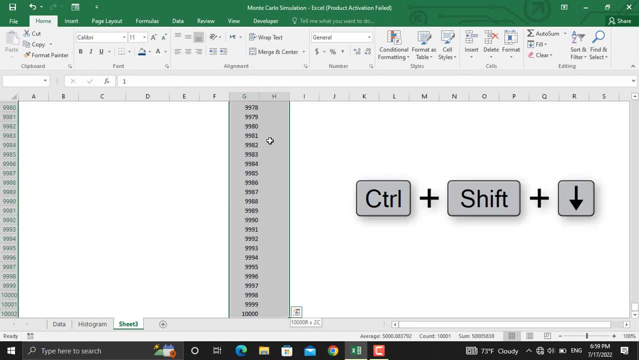 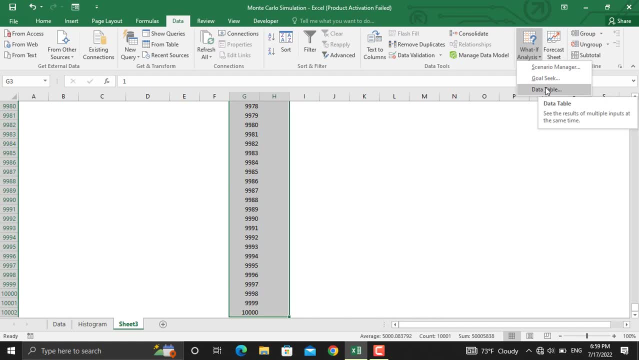 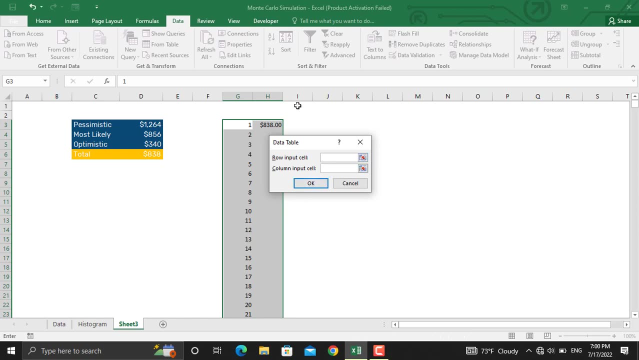 I'll hold ctrl, shift, right arrow key and down arrow key, then I'll go to data. from here I'll click what if analysis. from here I'll click data table and from here I'll leave the row input cell blank and for the column input cell I'll click. 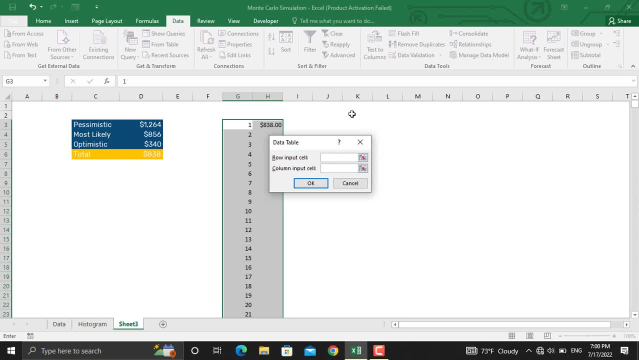 anywhere outside the selection. so I'll click this cell, click OK. as you can see, the probable cost for the risks will be filled in here and we have it up to a 10,000. now, as I have this area selected, I'll go to insert and from here, from the 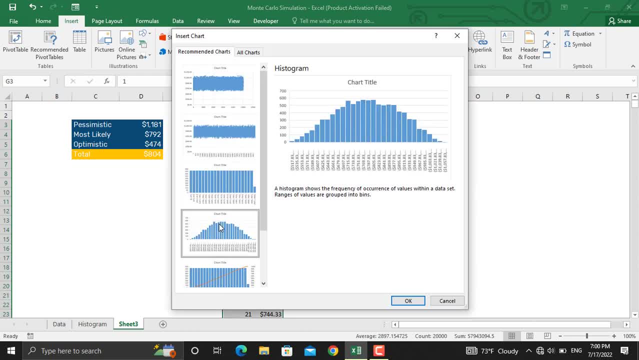 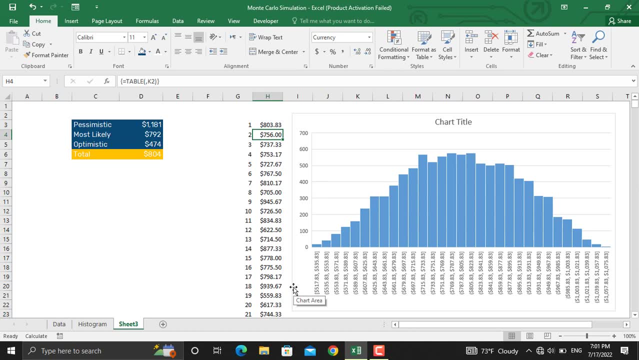 recommended charts. from here, I'll click the histogram for a Monte Carlo simulation. so this is how you can prepare the Monte Carlo simulation for quantifying the risks in your project. if you like the content of the video, don't forget to subscribe to the YouTube channel and hit the bell icon so that you don't miss any of my new videos. and don't forget to subscribe to the YouTube channel.